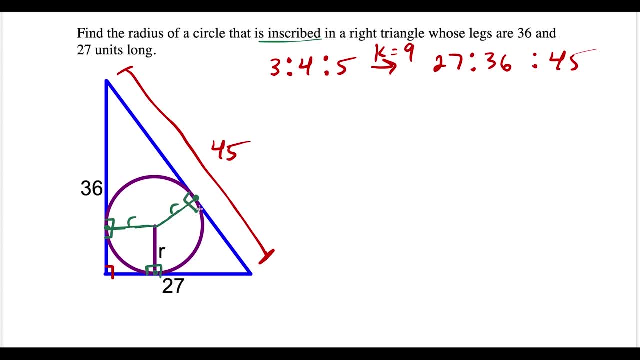 angle formed is 90 degrees. So I'm just going to draw in a few right angles like this. So now the next thing that jumps out at me is that over here we have a square because all four angles here are going to be 90 degrees. Since we have 90, 90, 90, the missing angle had to be 90.. And if all the 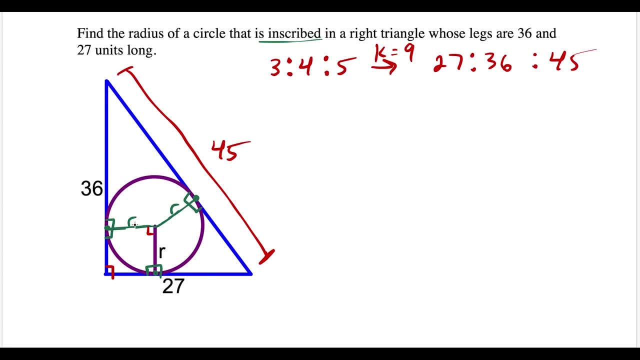 interior angles are the same. that tells us, for now, that we have a rectangle, but with rectangles, opposite sides are equal. So this would have to be r, and then this would have to be r. So now this is definitely a square, because it has all right angles and all four sides are equal. So now what we could do is we could express this: 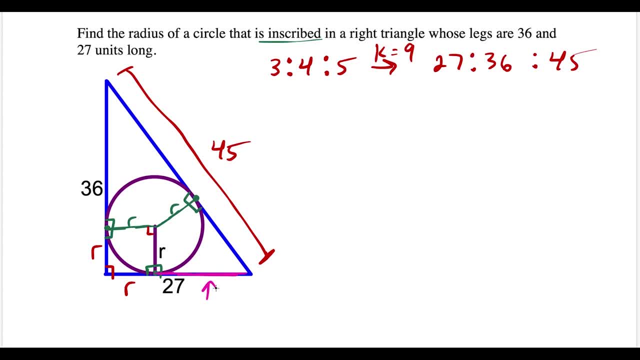 length over here. So I'm going to highlight this in pink: This length, if the entire thing is 27 and this is r, then this piece here we could call 27 minus r, Because once again, the entire distance from here to here is 27.. 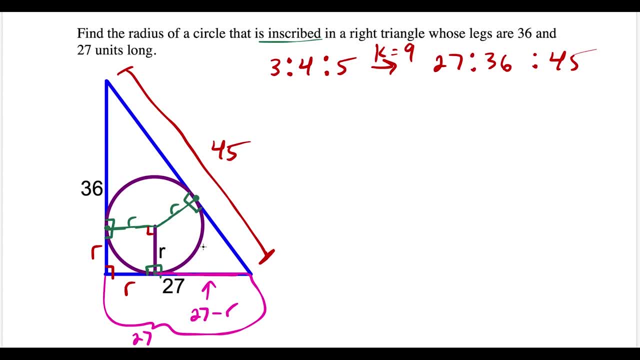 and is. this piece is r, so we would just subtract to get this distance here. but one thing that jumps out right away is that when you have tangents that are meeting at a common point, then these segments here are going to be equal in length. so this piece over here I can highlight is pink and this is going to be 27 minus r. 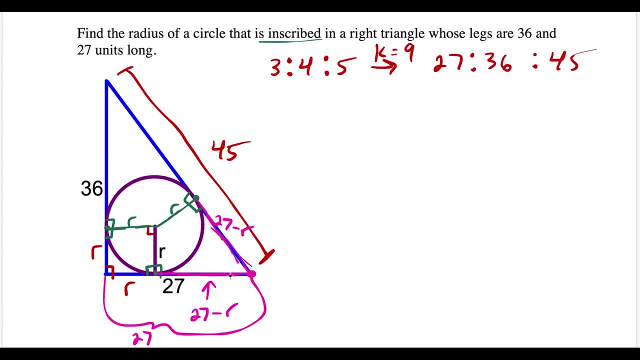 But let's say you didn't know that the tangents drawn to a common point are equal in length. What would we can always do here is we could draw this line in down the center like this And notice that these two right triangles are taken as the 128 steps because they're quite close together according to each other. they're in this first section. so again, if we runeros and we caninis, 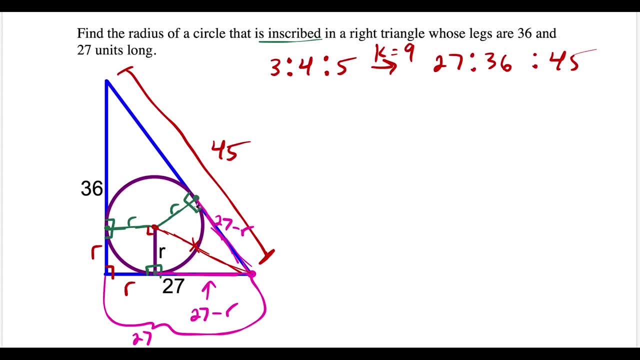 here share this common side like this and they have the same leg length of R. so you see how R is a leg in both of those triangles and they share the same hypotenuse. so by hypotenuse leg these two triangles here these two right triangles would be the same. so that means this pink segment here 27 minus R. 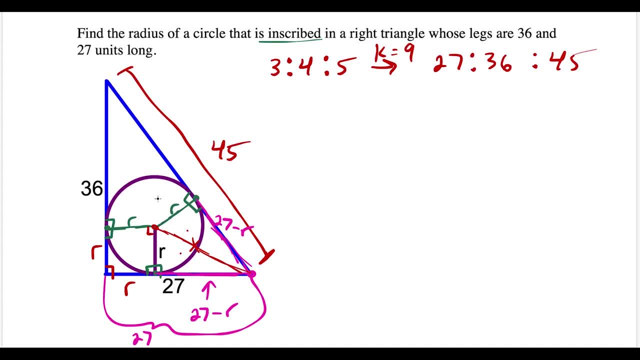 would match in both triangles, but now we'll just use that common idea for the rest of the question. so the next side I want to label here is: notice: this entire side is 36, so if this segment is R than just this piece here, that i'm 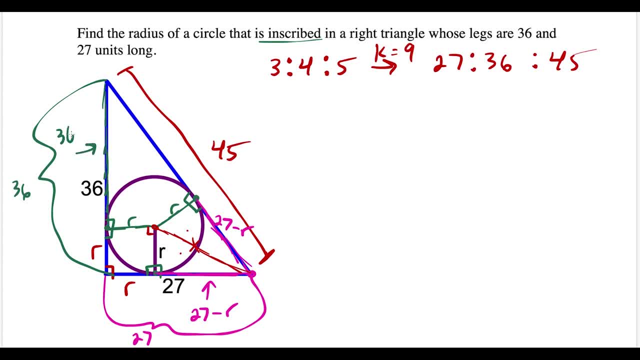 highlighting in green. that segment we could say is 36 minus R. but notice, we have two tangents here drawn to a common point. so this segment that I'm highlighting in green is also we could, something we could express as 36 minus R. so now we could just combine all of this information. what we know is that this: